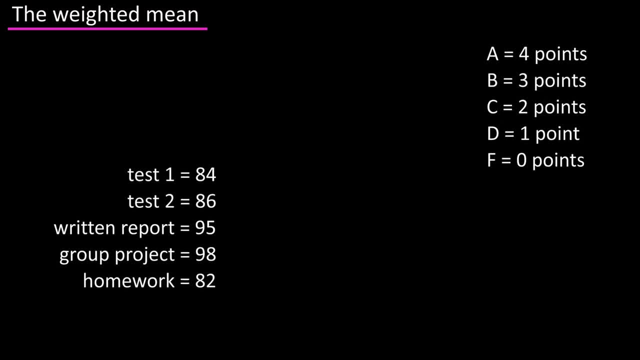 There are sometimes data sets where some values are more significant or have more weight than others. For instance, you may take a class where your grade is determined by five different things: test one, test two, a written report, a group project and homework. The instructor puts weights. 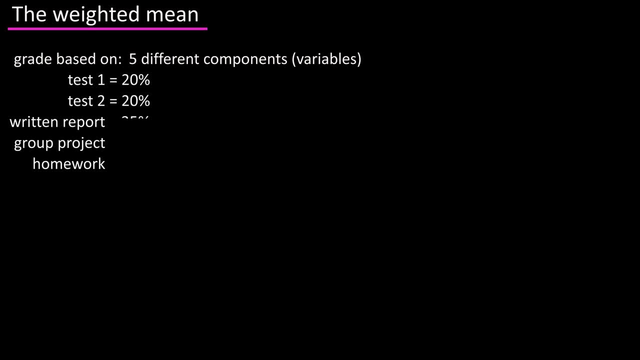 on these. Each test will be 20 percent of your grade, the written report will be worth 35 percent, the group project will be 15 percent and homework will be 10 percent. Your weighted mean will determine your grade in the class with the normal grading structure as you see here Your results. 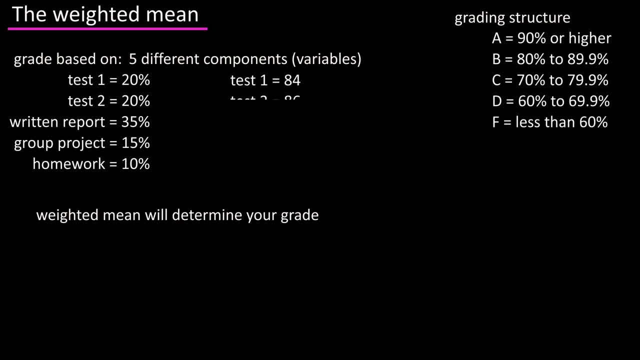 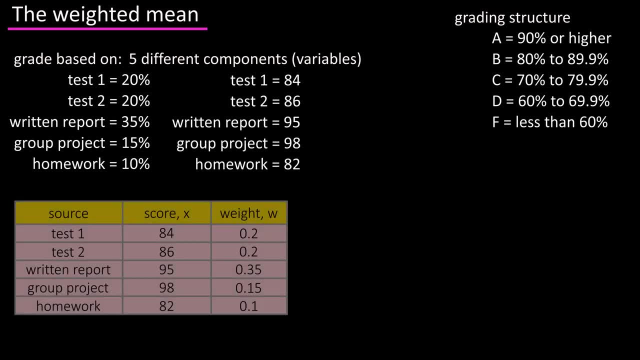 on. the five variables are 84 on test one, 86 on test two, 95 on the written report, 98 on the group project and 82 on homework. First, we're going to arrange our data in a table, with column one being 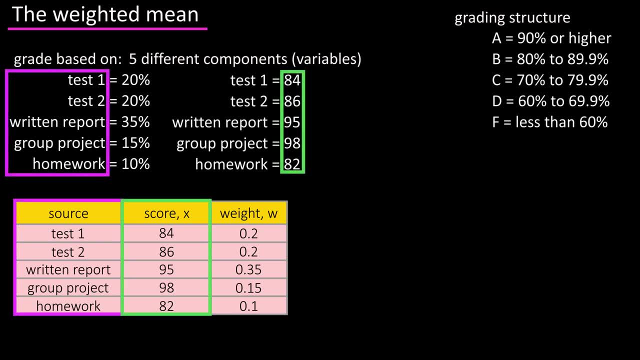 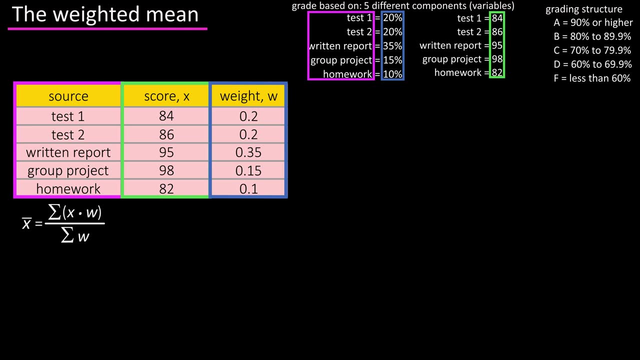 the source or variable, column two being the score you got, column three being the weight. so 20 equals 0.2,, 35 percent equals 0.35, and so on. The short formula for finding a weighted mean is: X bar equals the sum of X times W divided by the sum of W X bar. 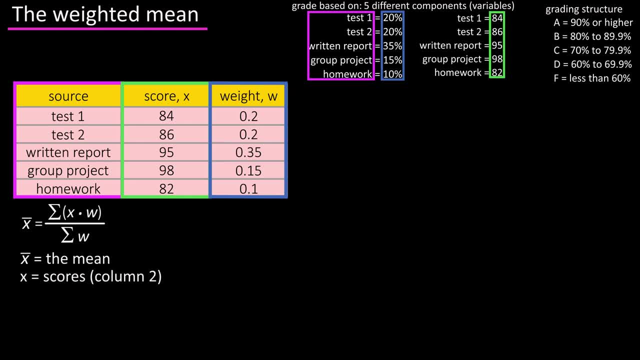 represents the mean, X is your scores from column 2, and W is the weight from column 3.. This symbol is the capital Greek letter sigma and it means sum of The long formula for this is X bar equals X1 times W1, plus X2 times W2, plus X3 times W3, and so on through X5 and W5, since we have five. 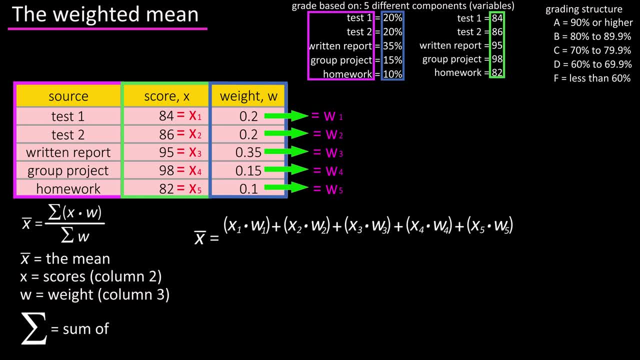 variables or sources. And if there were more sources or variables, this would continue on to how many other variables there was, And the bottom of the equation is W1 plus W2 through W5.. And if there were more sources or variables, this would continue on to how many other variables there was. 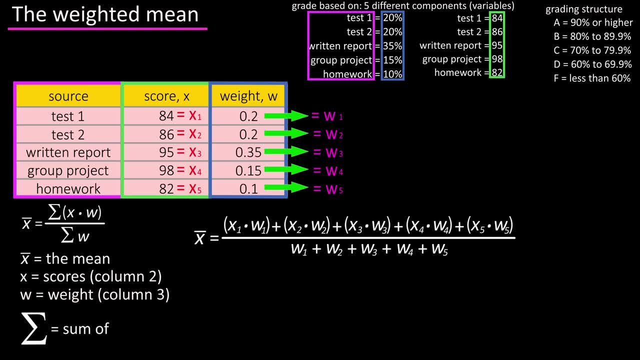 So the short formula makes it more compact. In our example, X bar equals 84 times 0.2 plus 86 times 0.2 plus 95 times 0.35 plus 98 times 0.1. Plus 82 times 0.1, which equals 90.15.. And on the bottom we have 0.2 plus 0.2 plus 0.35 plus 0.15. 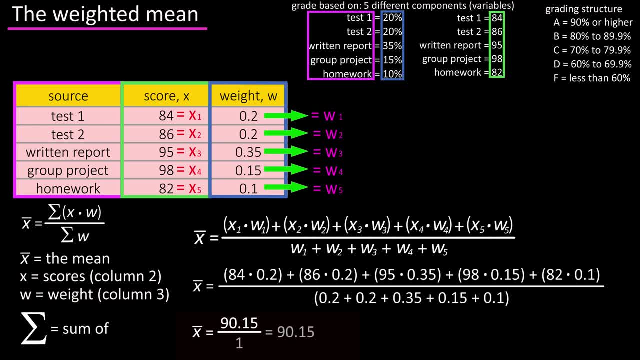 plus 0.1, which equals 1.. So 90.15 divided by 1 is 90.15. And that is your mean. So your grade in this class is an A. There's actually a quicker way to find the mean: We can create a column 4.